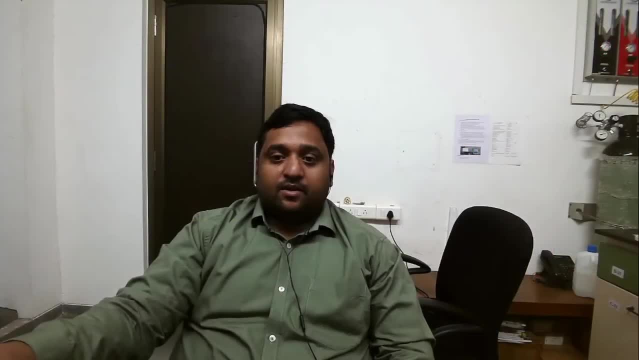 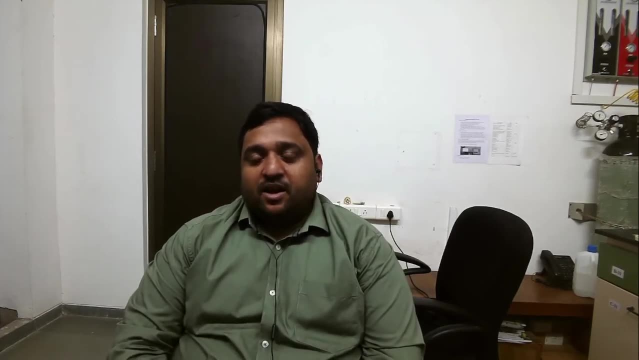 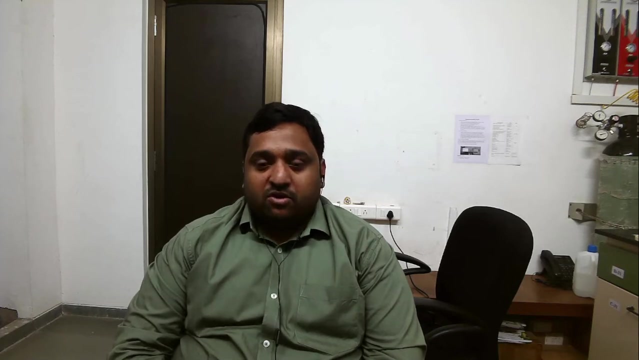 Hi students, welcome to my lecture series on process plant operator and if you, if you would have followed my earlier lectures and you might have learned the following things: that on off control systems which will be used for the, we discussed about the level control, temperature control. it is a kind cheaper process. then we come back to the. there are two videos that 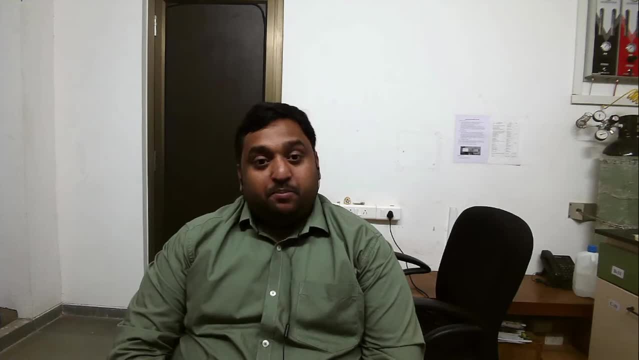 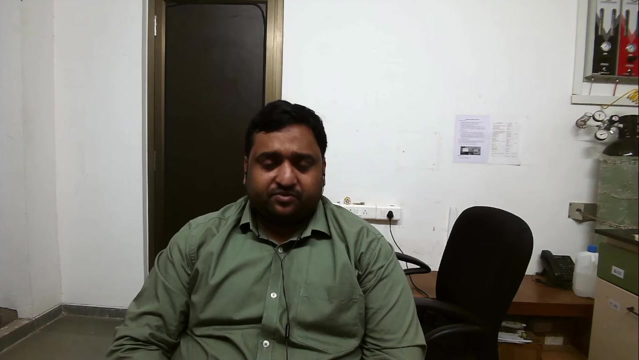 are uploaded based on P and PI controllers in the systems. Now you are acquainted with the controllers and continue to what we have learned. for the P and P IP ID controllers, We are going to see a simulation based on how people will maintain the pressure in a vessel in a process industries. okay, we. 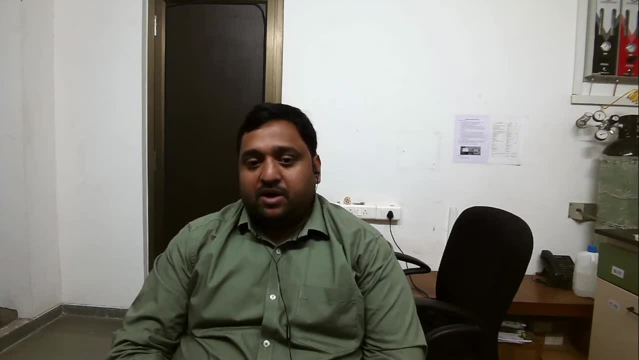 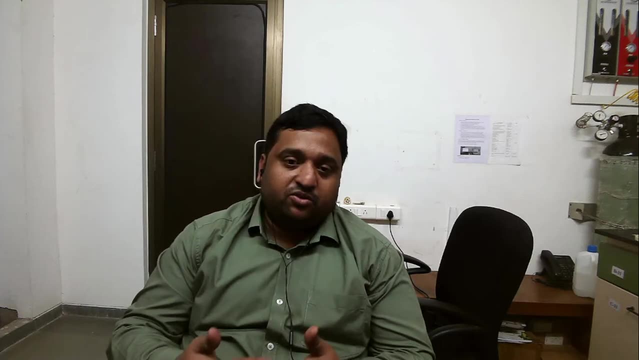 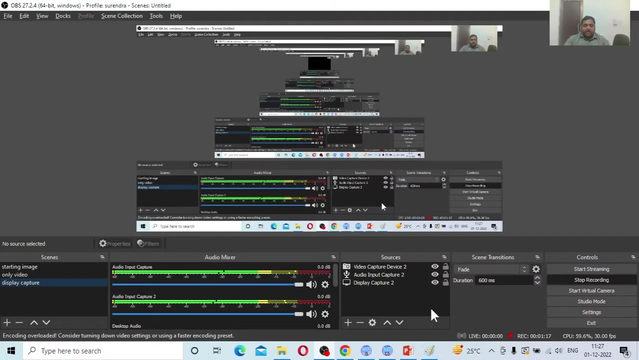 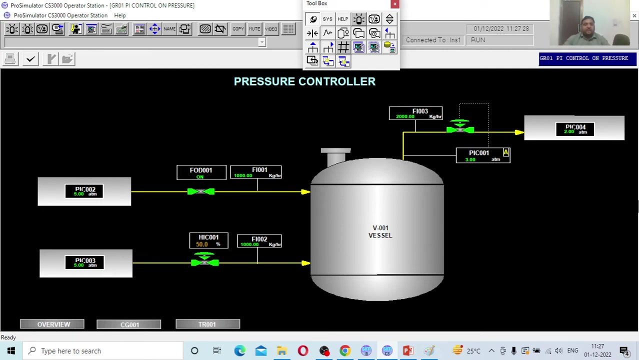 are going to show you. I'm going to show you- I mean on a simulator platform, those who people watching for the first time. I request them to follow the earlier lectures so that they will be more acquainted. let me go to the simulator. this is how a graphic window of pressure controller looks like and the main. 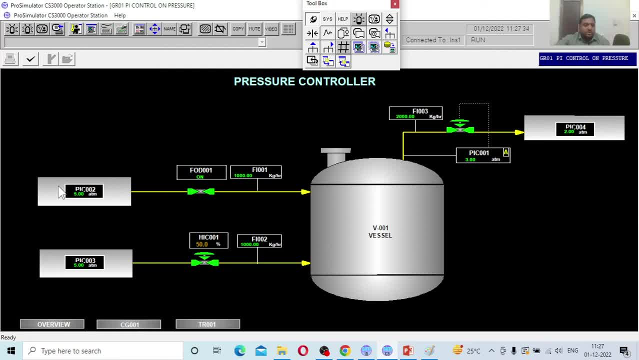 important for the pressure controller is to maintain the pressure in the vessel. so the job of maintaining the pressure in the tank is controlled through this control valve and we know the basics, that how the controller receives the signal and what how it is in general kind of signal it generates and it goes. 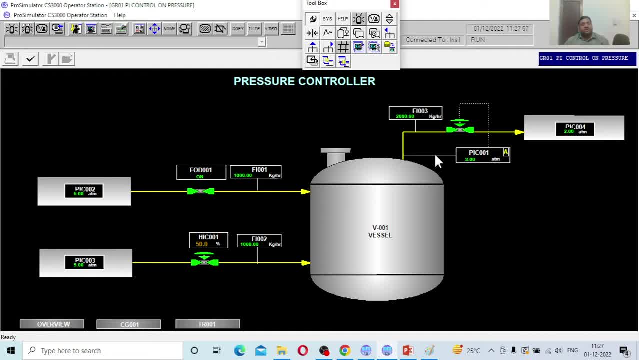 to how the pneumatics- I mean how the current signal- is going towards the pressure signal, so that, ultimately, this valve will be controlled. okay, That is it. This is some process line. There are two process lines, and PIC 002, 5 atmospheres, and PIC 003, one of the which 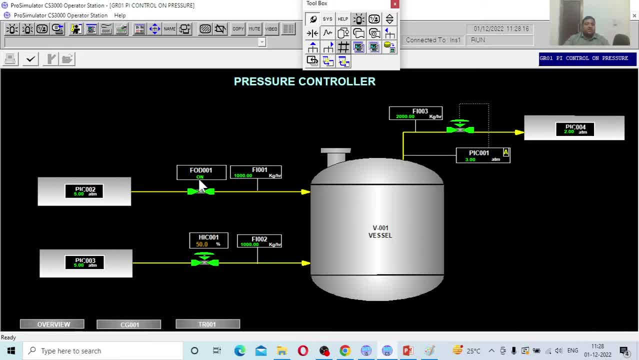 the edge stream coming at a higher pressures. okay, through this non-return valve. okay, This is a non-return valve FOD flow of direction. I mean FOD represents that is okay. And one line is having the flow rate of 1000 kilogram per hour and second line is also: 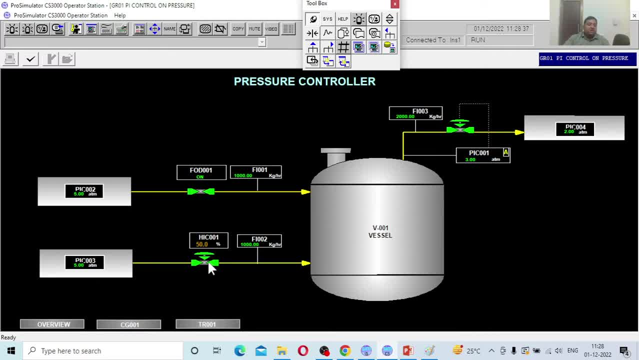 1000 kilogram per hour, but it is coming through the manually controlled valve. okay, Now the present, this manual control valve is 50 percent open And this is the vessel in which they have to maintain the pressure of 3 atmospheres, because the pressure, the line, the pressure, in this particular, both the lines- are 5 atmospheres. 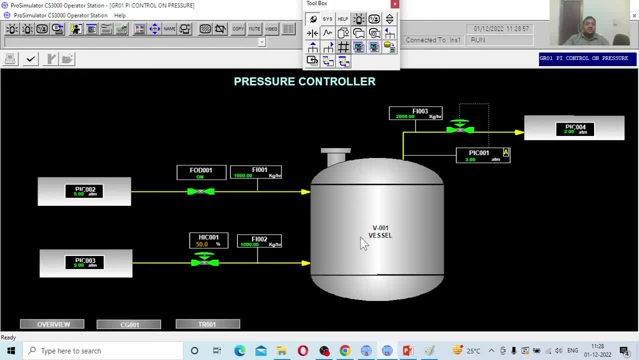 but there is some utility that is required at the 3 atmospheres. That is why they have to maintain the pressure in the vessel around 3 atmospheres. you can see, Yeah, Presently the flow exit to the flow. of course it is at the steady state. 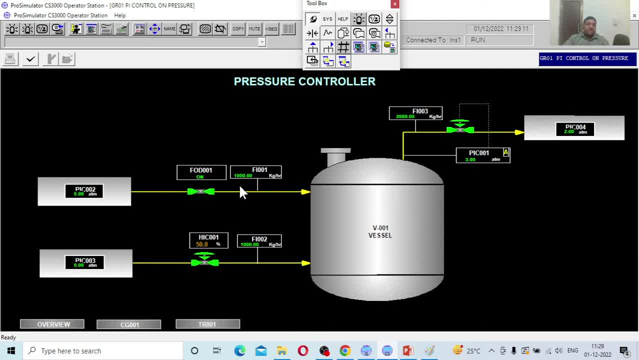 The flow outlet to the flow is 2000 kg per hour, which is a summation of FIC FI 001 and FI 002.. And if, at the moment, I click the controller, I am going to open the pop-up window that. 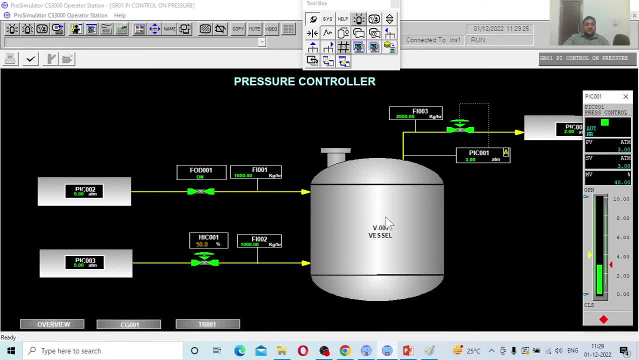 okay, Present the process value. that means the present process, I mean pressure inside the vessel is a 3 atmospheres. I have also wanted to maintain the 3 atmospheres in the particular vessel. both are same. To maintain this pressure in the vessel, the valve has to be open 40 percent. 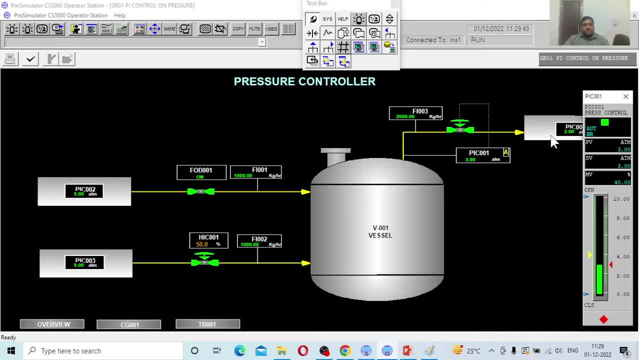 That is what the, because exit pressure is a 2 atmospheres. okay, Presently you just do not worry about this because there is a imagine. there is some flow that is going at high pressure to low pressure through this vessel. Okay, 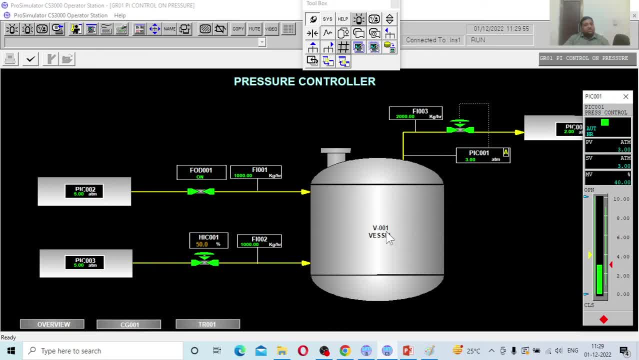 Okay, So the vessel has to be maintained at 3 atmospheres because the stream that is coming at higher pressure, it has to be controlled one. So the sensing element at the exit of the particular vessel will give a certain signal to the controller based on the pressure. automatically the valve will be controlled. 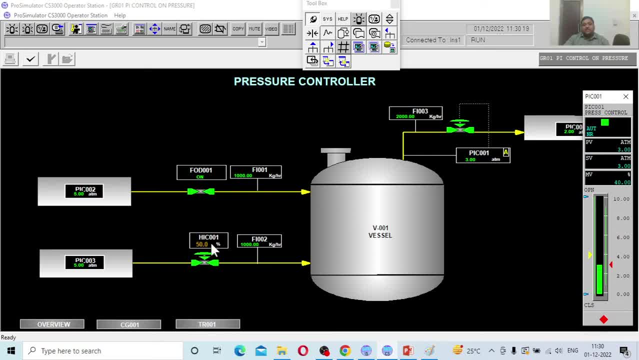 Example: if I open this particular valve, HIC 001, to a higher valve position, what happens? The flow to the vessel will be increased. okay, If the flow to vessel will be increased, the pressure is going to rise. okay, The process value, which is a presently 3 atmospheres, you can see now, because of increase in flow, because at high atmospheres the pressure inside the vessel will increase for a moment, But that pressure has to be controlled. to come back to the 3 atmospheres, which is the controller does the job. That means it receives the signal of the increase in pressure based on the control. 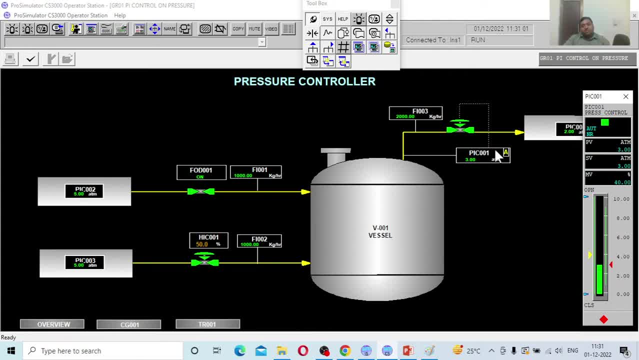 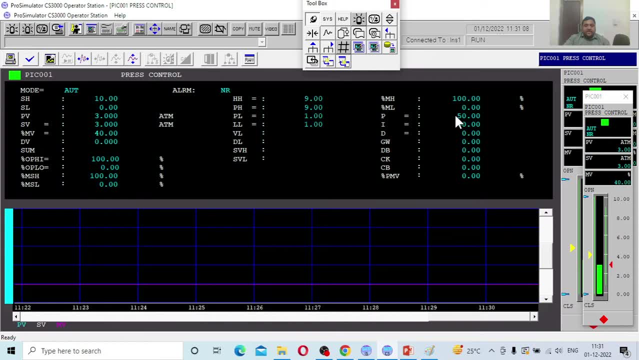 action is going to takes place, What kind of controller at this moment they were using? Let me, if you go to the PID controls and, as I can see, P is 50 and I is 60. That means both are at a lower values. 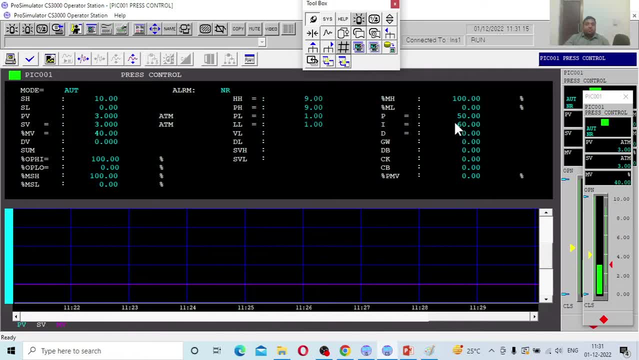 That means it is a kind of PI control systems. If I put 0 at I position or higher number, automatically this become only P controller. I have already discussed about there are issues with the PID. Okay, That is why in industries at the control never come with a P controller either it. 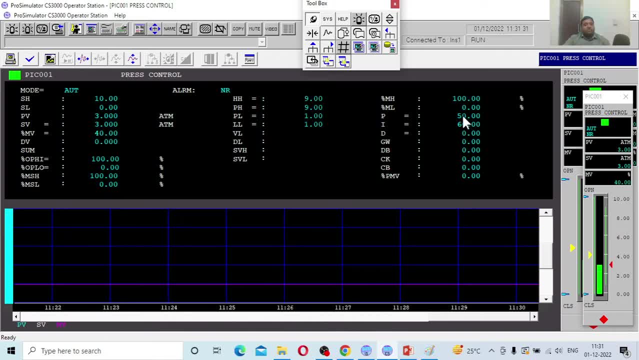 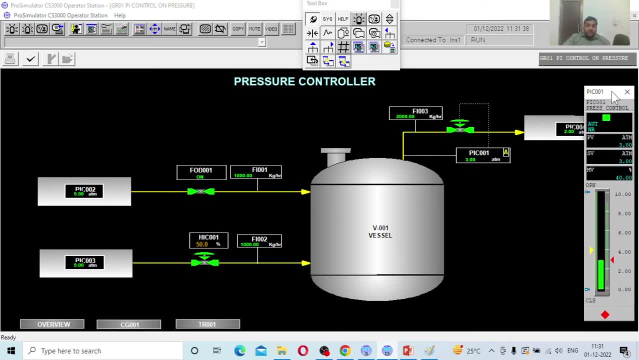 is PI controller or PID controller. So you have to remember this. okay, let me go back to the graphic window. So the moment now you observe what happens. the moment they open the particular valve- 50 to 60 percent the process value here is going to be changed. 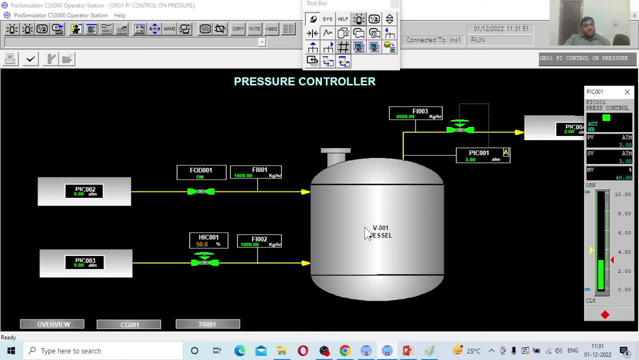 Accordingly, if high flow is going into the system, what the controller will do? Try to increase the valve position. presently the valve position manipulated variable is around 40 percent. So automatically, because of the increase in pressure in the vessel, immediately the 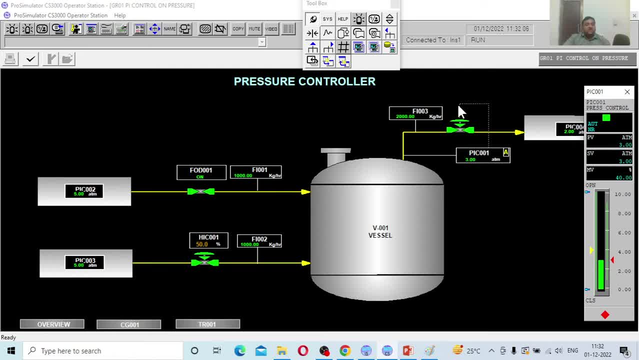 controller will take the action to open this valve. okay, because now process value and set value are different. Let us see. I am going to open this valve. imagine, see the things that are happening. okay, One second, I will put it here. 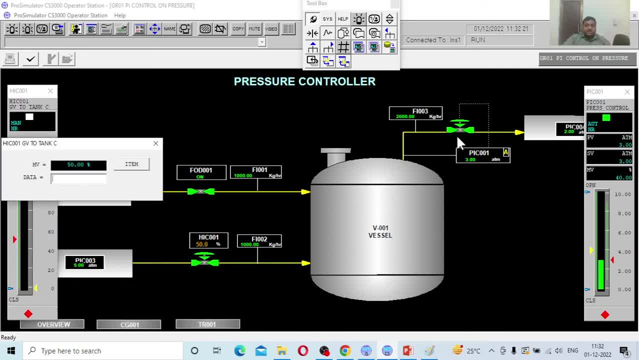 The moment I valve. observe this lines, observe this. So I am going to open this valve. Okay, Let us observe this. okay, See the flows. okay, 1000, this is 1000, this is 2000.. 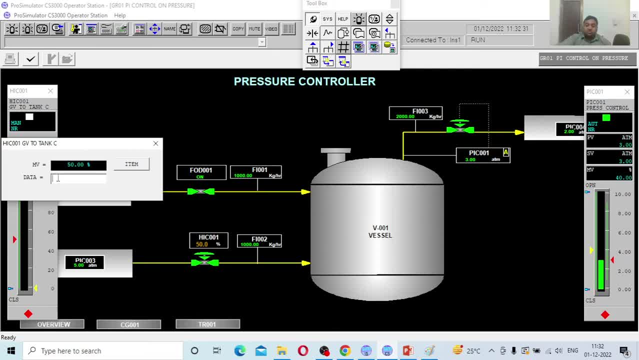 See the set value, see the process value. everything you have to observe. See now I am opening the valve- I mean hand indicating control- to 60 percent. Suddenly the flow has raised into the system. suddenly the pressure has been raised- 3.1,. 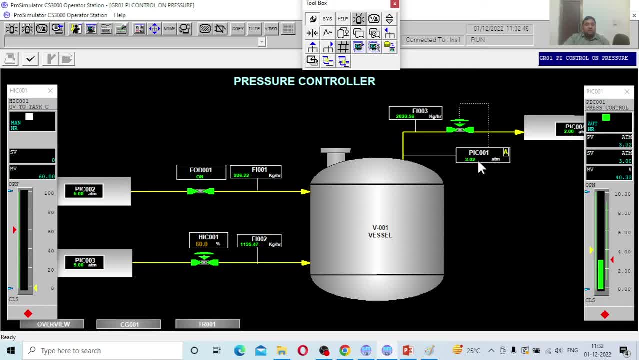 which is greater than the set, Immediately the controller will does the job of bring back to the 3 atmospheres. that is what, How it is going to work. Now you can see earlier it is manipulated: this 40 percent, now it is 40.6,, 40.626,. why? 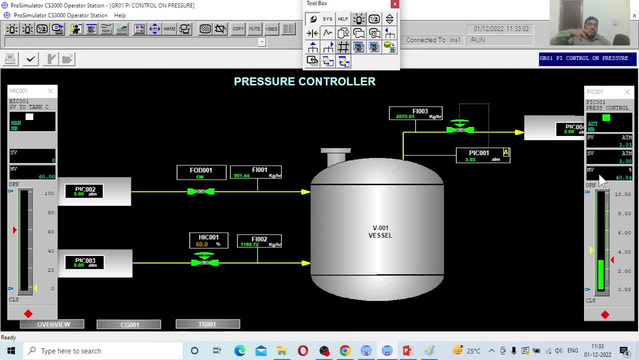 Because there is increase in flow, the valve has to be, now it has to be at a higher position. Earlier it is 40,, now it is 40.9,, 41,, 42. See, it is trying to adjust the pressure by increasing the flow from the vessel. okay, 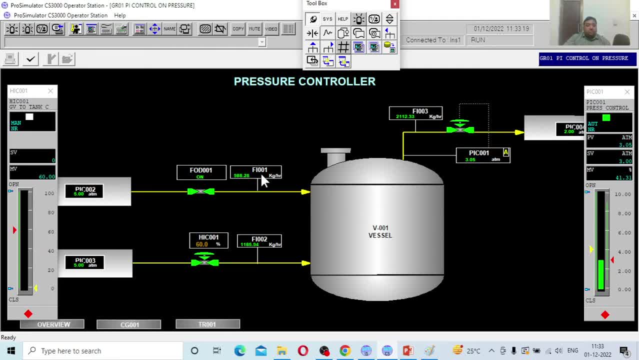 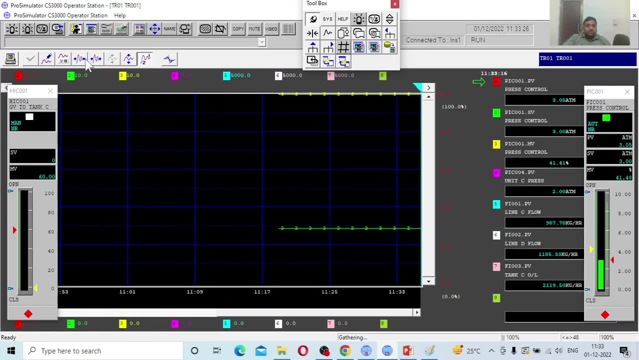 Now you see it takes time. Now if you go to the trend window: okay, Now you see it takes time. Now if you go to the trend window: okay, At trend window, you observe, you can observe, okay. 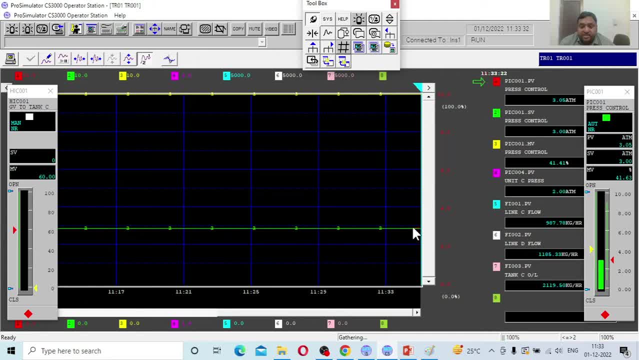 This is now we can see the slightest disturbance that happened. Let me remove this manipulative variable for the moment and try to. yeah, You can see the present process value and the present value. Now, if you see, the color code is also given. 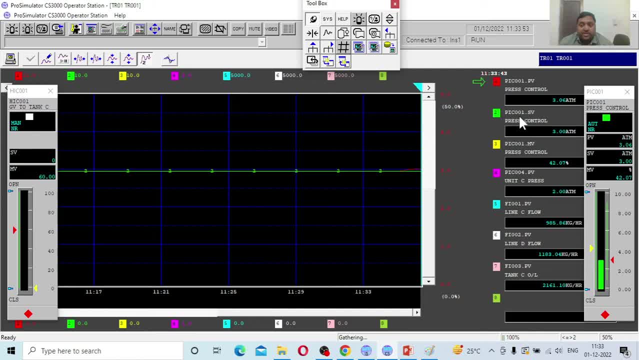 Okay, This color is number two is indicating, you know, set value Number. this color is indicating the process value. Now you can see the slight increase because of pressure was raised. the process value increased because of the disturbance that is given to the system. 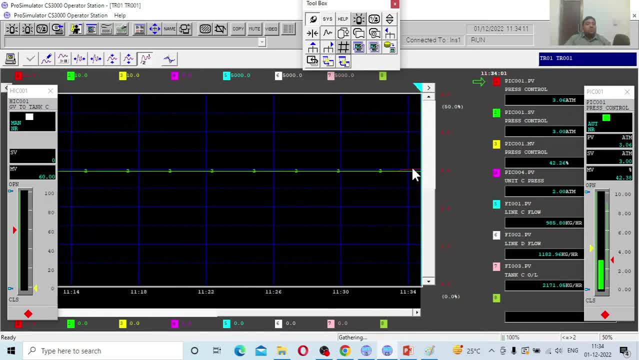 Automatically, a slight increase in pressure has been taken place. Now what the controller will do: Try to bring this high increase in pressure by to the set point. okay, That is what the controller will do. That is what. see the difference. now it is going to get reduced now. 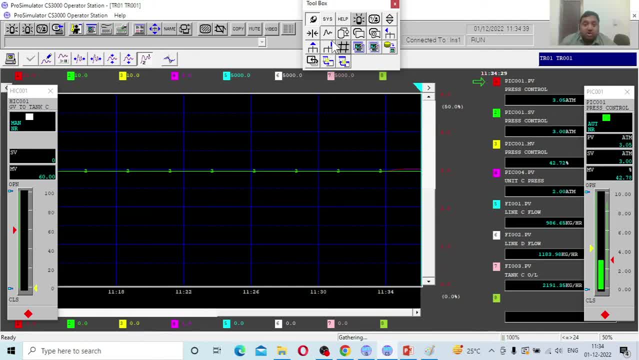 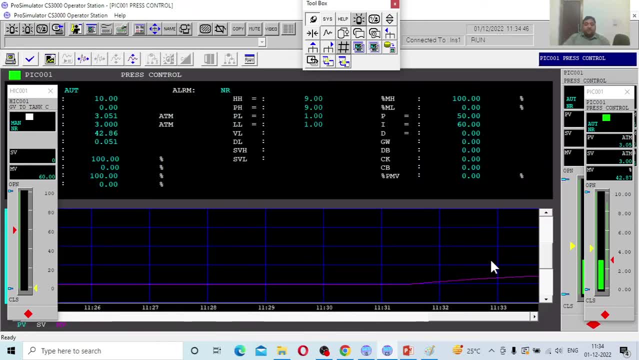 Even though if I go to the controller in window, let me go to the control window. you will be more clear. So see the difference. If you observe here the pressure was raised because of the increase in flow. that happened because I have opened the valve slowly. it is raising now the controller is will bring. 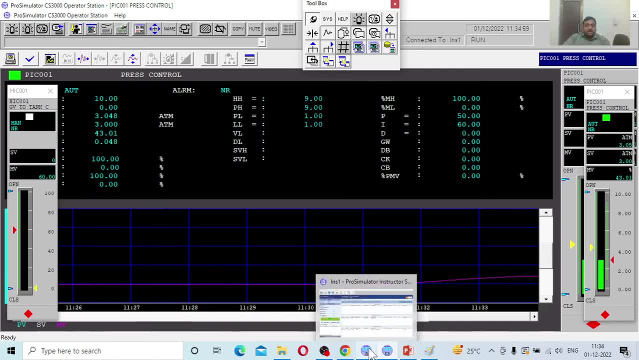 back to this particular set point. Let me speed up the time 5 times so you will observe more trends. see what happens Now you can, which is a short period of time, though. now the set point will try to match with that of a process value. 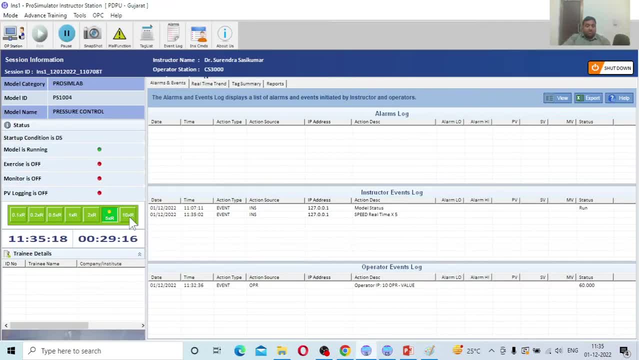 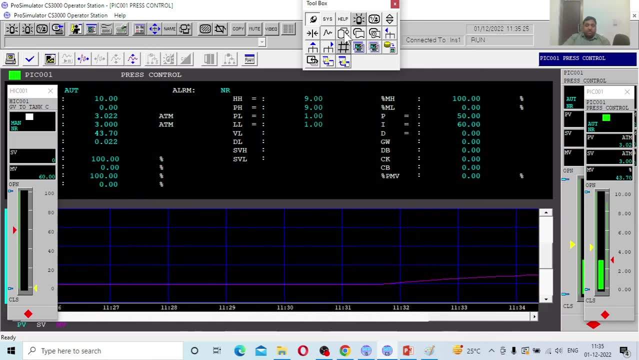 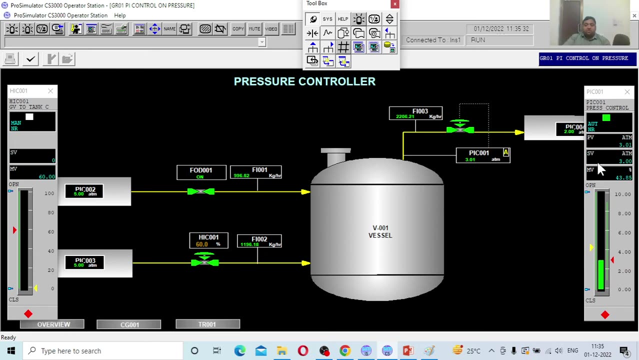 Let me order of the time, go 10 times. Now, if you go to the graphic window, see now the set point process value is 3.01, now the set value is 3.. So slowly now the process value will be matched to that of a set value, even though even the 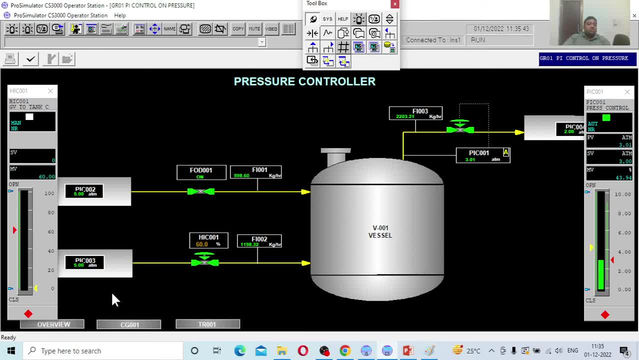 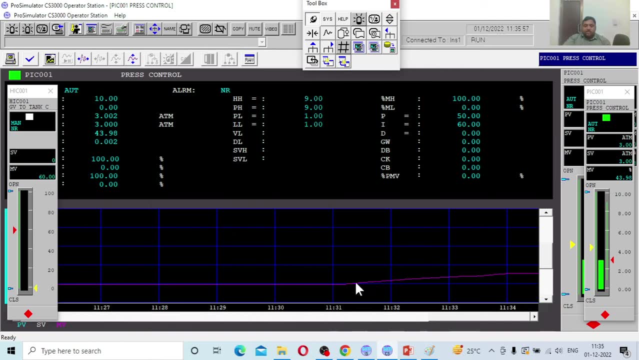 smallest raise in, I mean pressure. that happened because of the increasing the flow automatically the control. Now you see process value and set value. both are matched. This is the beauty of the controller systems. let me, it will going to happen soon, so now. 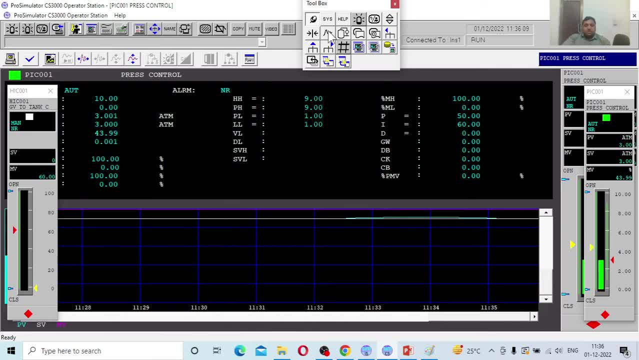 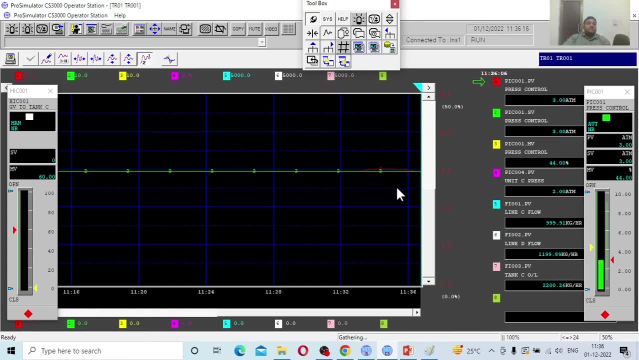 both lines are getting matched. If you go to the trend window also, you are going to observe. See, there is a small hump earlier. now this hump is getting reduced. Now the process value and set value are matched. This is the first thing we can observe. 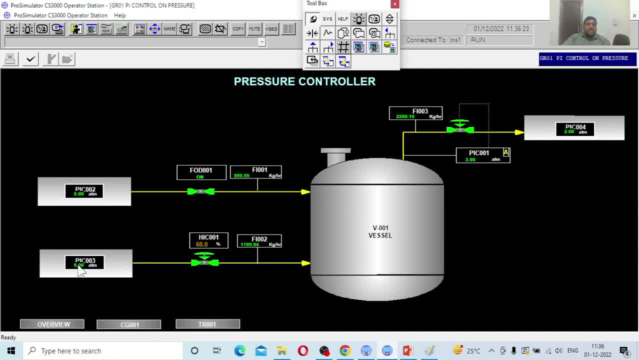 And what are the other things we can observe. This is called servo problem. servo problem means there is a disturbance we have created and the controller will take action to reduce the disturbance. that is called servo problem. And the second problem we can discuss- I mean this is called, not servo problem. this is. 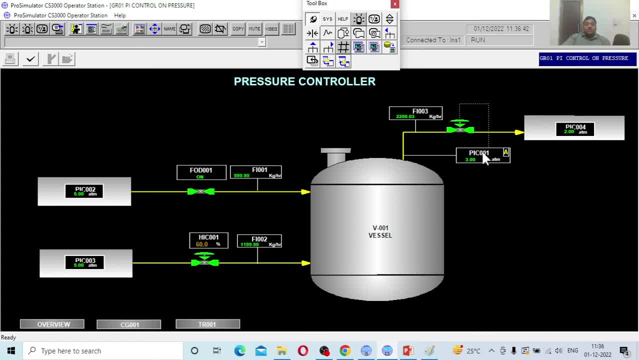 called disturbance problem. Now let us go to the servo problem. that means now I wanted to change the set point. Now the tank is maintained at 3 atmospheres. I wanted to maintain this tank at 4 atmospheres. earlier we have discussed that is called servo. 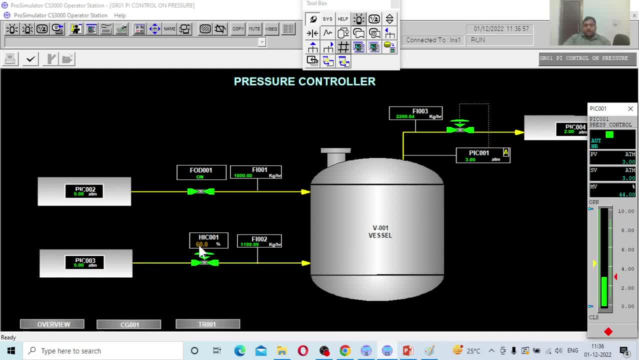 problem. Now we have, I mean disturbance problem. now it is servo problem. See, now I am going to increase the set point. now See what happens everywhere. I wanted to maintain at regulatory problem. yeah, I was not striking to my mind. 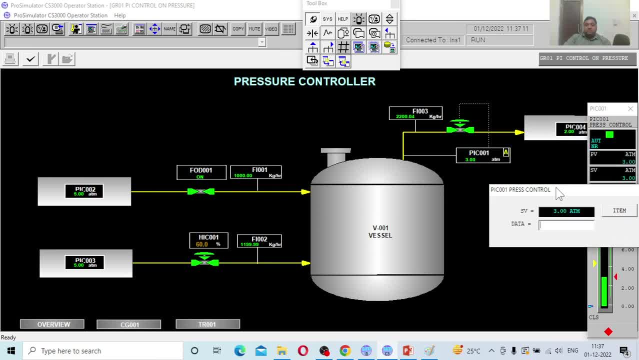 This is called regulatory problem. now we are going into the servo problem 4.. I wanted to maintain this tank to the 4, see what happens. See the manipulated variable earlier. it is 40, that is if I wanted to maintain at higher.